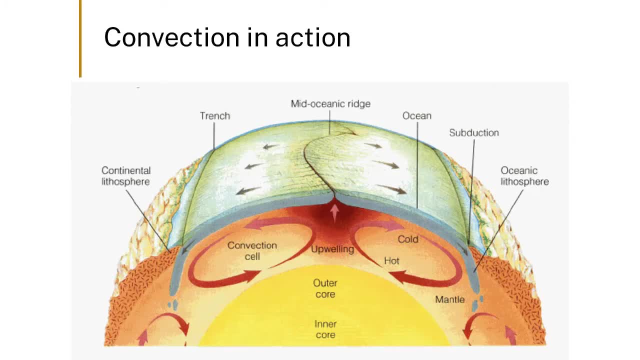 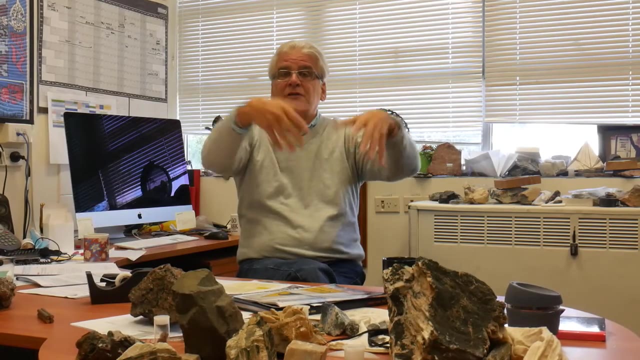 is when basalt comes down, it melts again, right, So the energy that it takes to melt, which is an endothermic reaction, we have to put energy in there. However, the opposite is, the exothermic reaction is when they come to the other end, they release a lot of that. 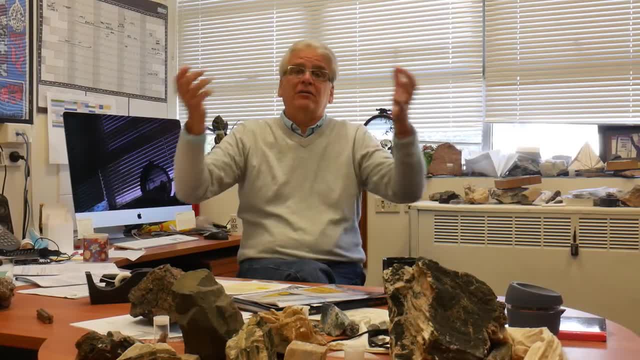 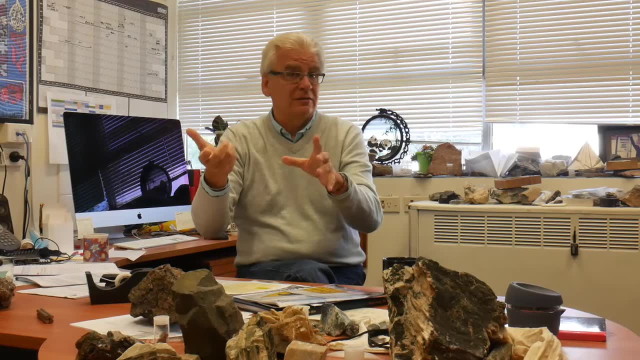 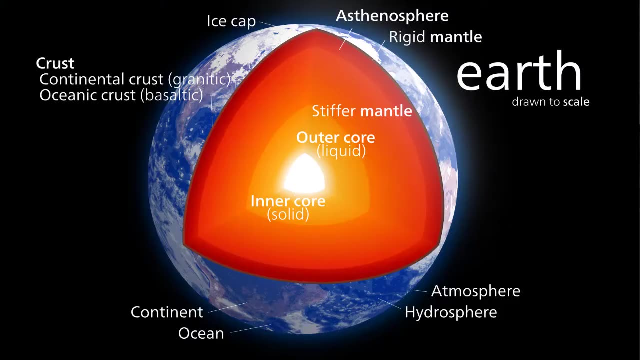 energy, So that we're transferring energy around. right, We have that original thermal energy, but then we're moving it around and we're switching between phases. So now the two biggest thermal effects on Earth are this really hot core and this cooling mantle? 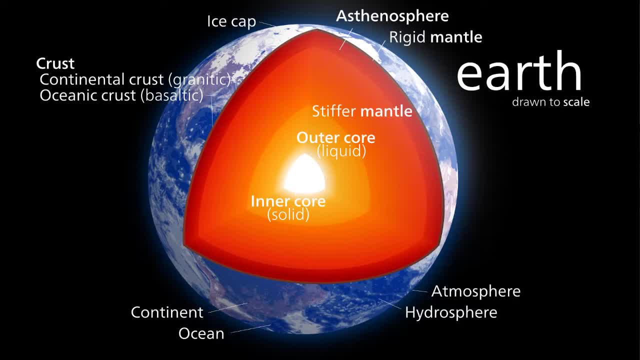 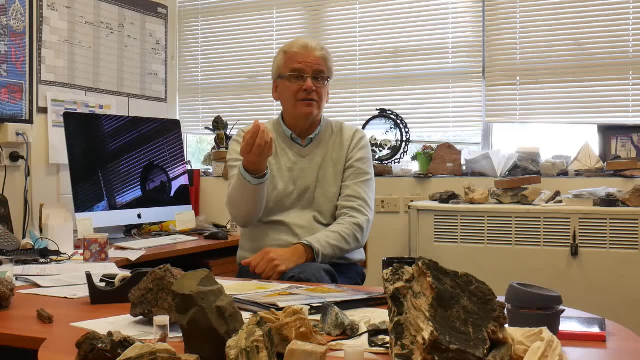 and so that there's a geothermal gradient as we go down, so that the places that we see heat coming out of the planet are where plumes arise, at mid-ocean ridges and at the volcanic arcs where the magmas are coming out. 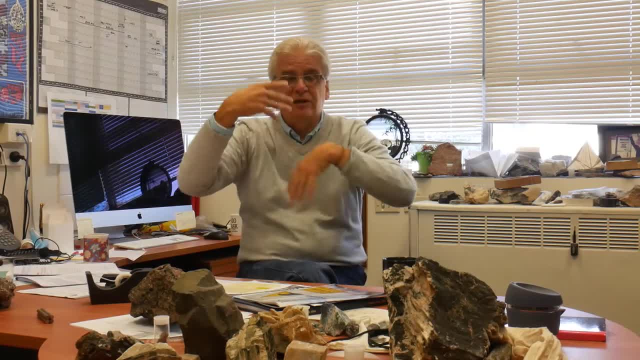 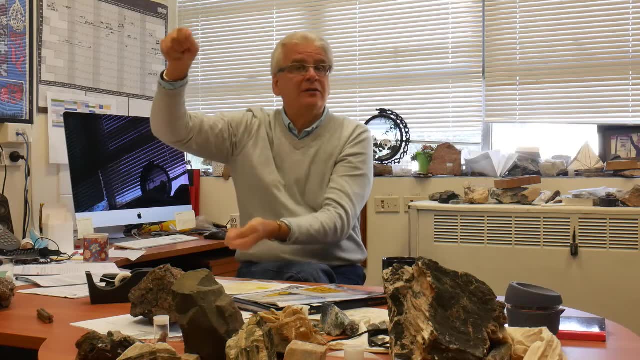 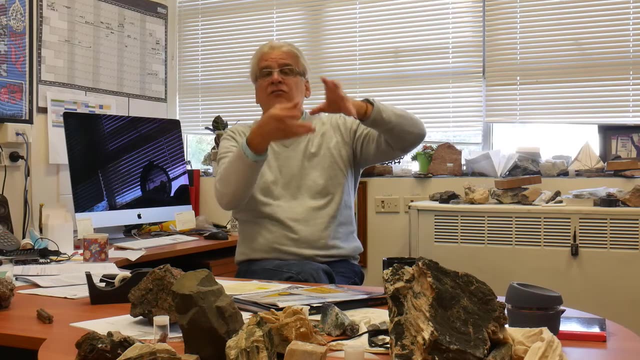 And so this is an interesting interplay between formation of crust, destruction of crust, building continents via that arc magnetism. When I say arc magnetism I mean above the seduction zone where the water comes out into the mantle flux is melted and that rises up. 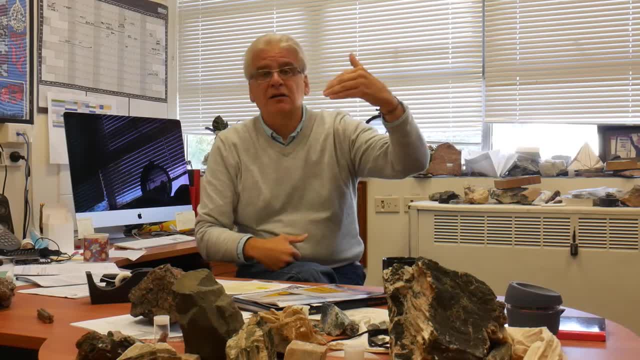 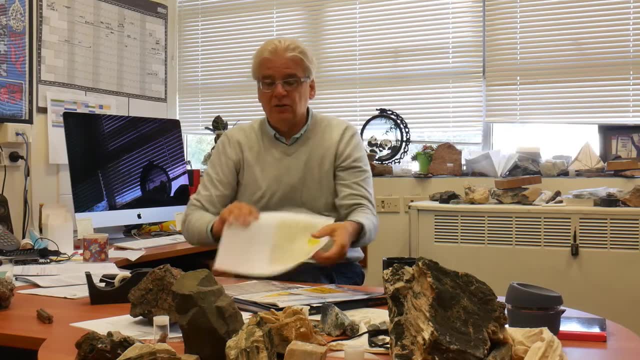 So we get chains of them and they're shaped like an arc because we're on a spherical planet And so the slab isn't like we draw. We draw, We draw the slab going down like this, but it's not because we're on a planet. 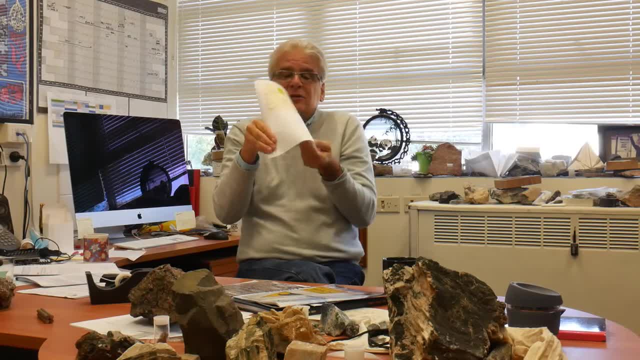 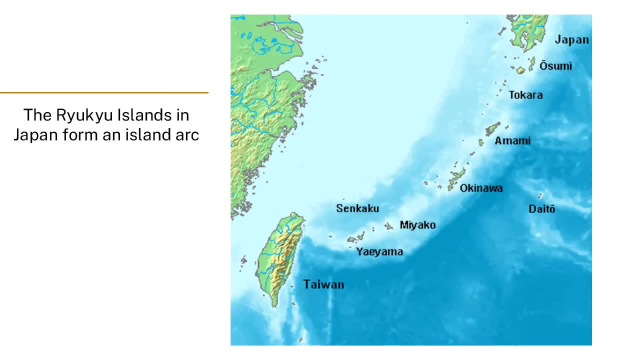 We're on a sphere, So it's going down like that, which means that it's an arcuate shape of the volcanoes that it makes. So if you look at the Japan arc, it's shaped like that, and all the arcs on Earth are shaped like that. 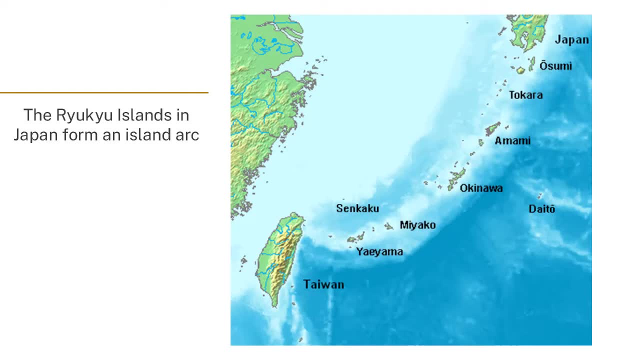 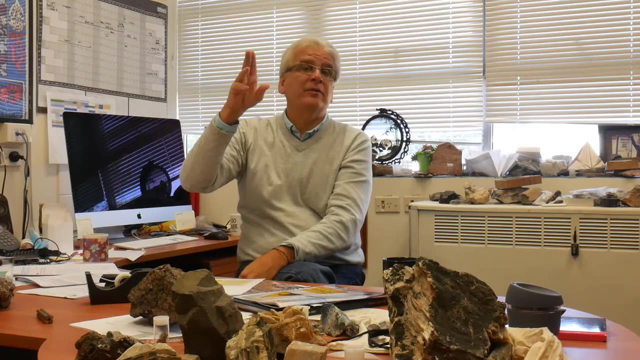 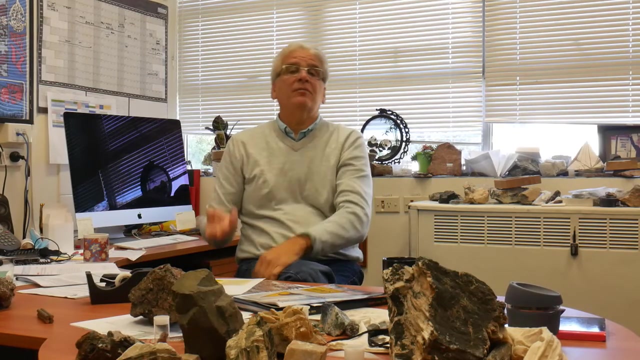 And the magma that forms from the dehydration of the slab, causing the mantle melting. it doesn't know what's above it. So it can rise up and come up, like Japan, in the ocean and make an oceanic arc, or it can be like the Andes and come up through the continental crust and actually help make a big mountain range. 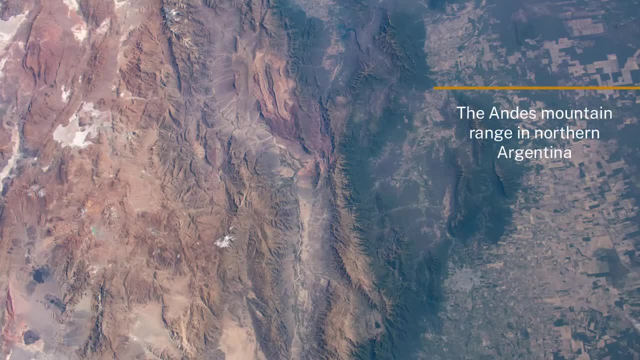 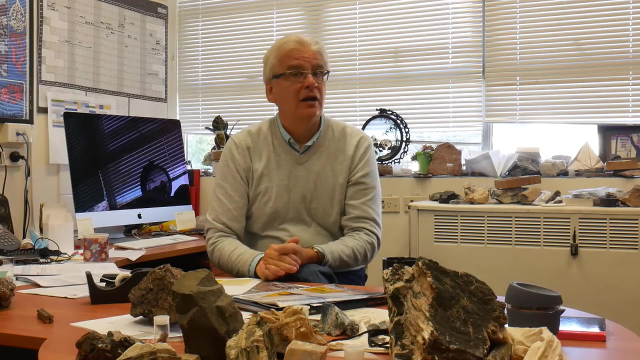 So we find the mountain ranges at the boundaries of the plates, And so either if it's ocean-ocean or if it's continent-continent, that's where we make the mountain ranges. So the mountain ranges are important in this whole process of reshuffling things around and moving them around.